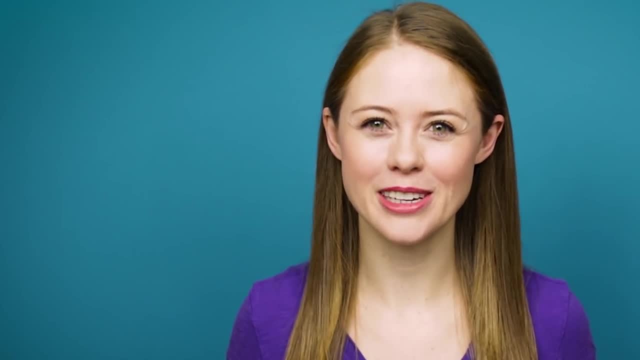 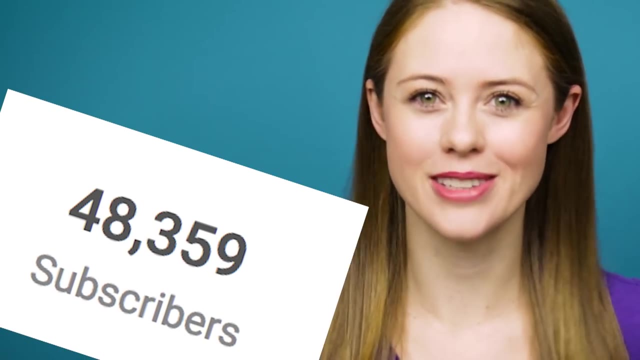 Hello Brains, Next week will be our one year anniversary. We have come so far This year. we made over 50 videos, we got over 2 million views on the channel and we are so close to hitting 50,000 subscribers. in our first year, We won YouTube NextUp. we made a two-hour glitter jar. we dealt 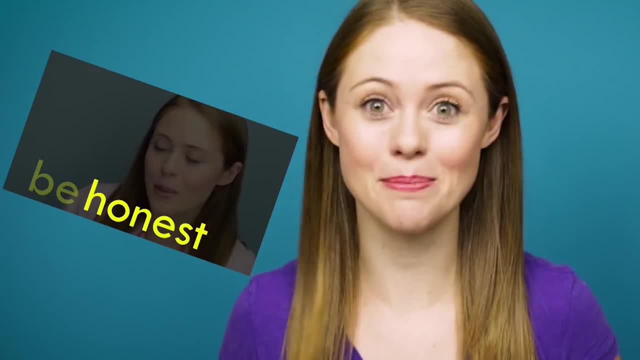 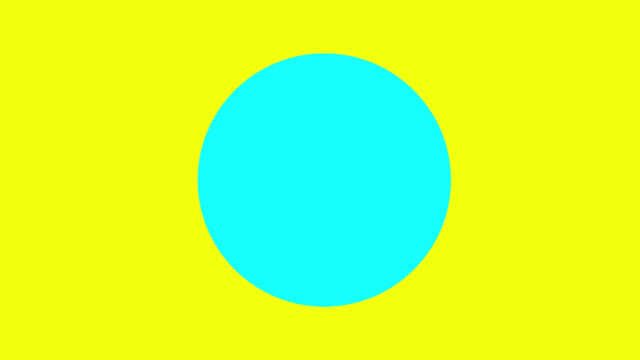 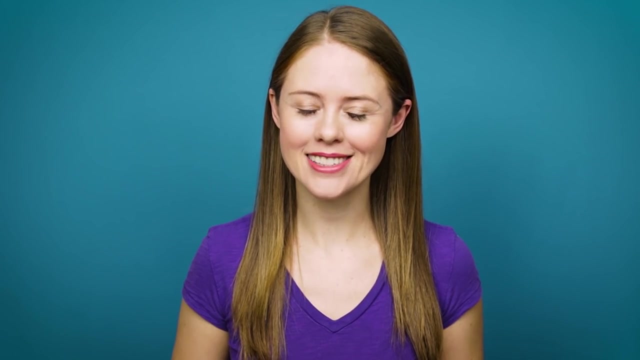 with meltdowns and procrastination and studying and relationships and paper clutter and sleep. What's sleep? Getting stuff done is great but, as I'm learning, it's also important to manage your time so that you're not up till 3 am every night. After a year of doing this show, scheduling is still. 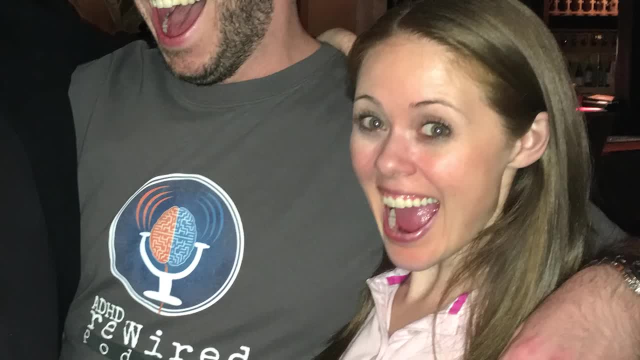 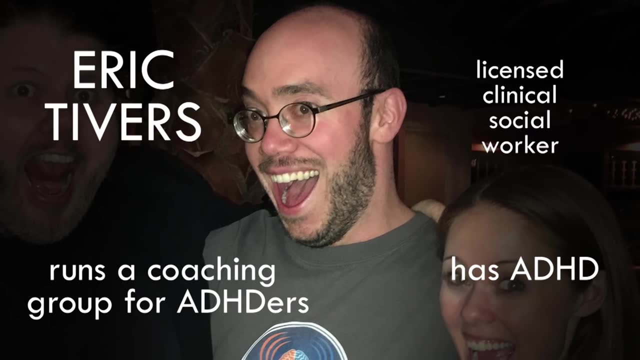 something I really struggle with, so this week we're getting professional help. This is Eric Tivers. He's a licensed clinical social worker, has ADHD himself and he runs an intensive coaching group for people with ADHD. He's also the host of the ADHD Rewired podcast, which you may have. 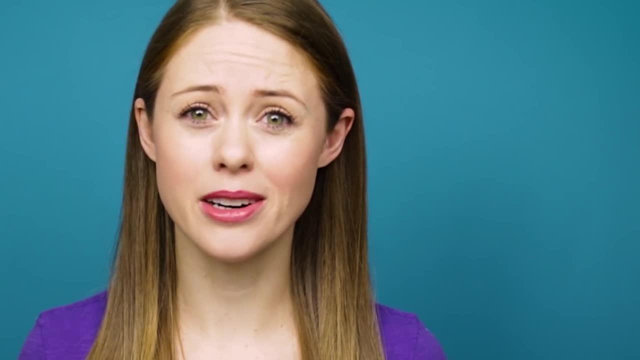 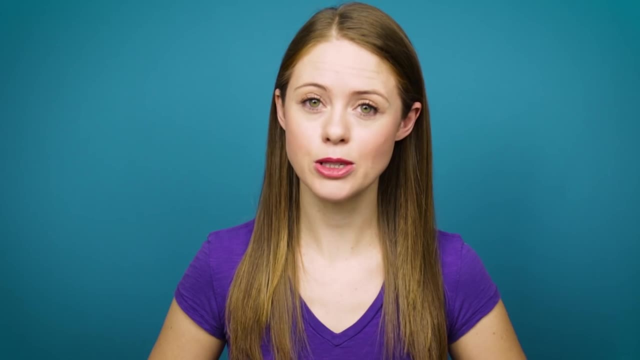 heard me on Link's in the description. Eric is also an all-around amazing guy, a good guy for doing this interview, even though I showed up 20 minutes late. Did I mention I filmed this from home? I was 20 minutes late to my. 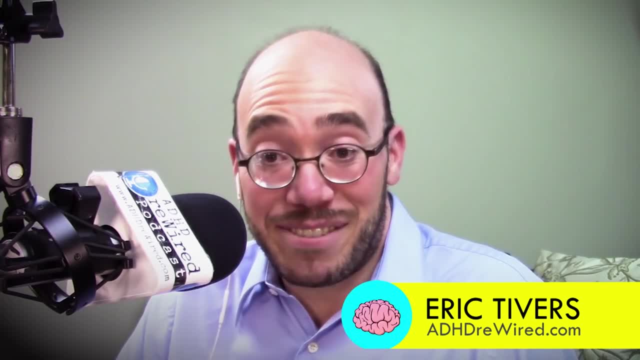 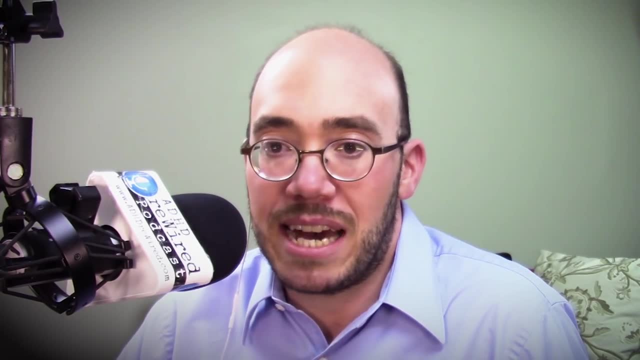 dining room. Thank you so much for coming, Eric, Thanks for having me. I'm really excited to do this. Help, Oh, that's my cue, huh. Okay, when you think of a schedule, what is that to you? 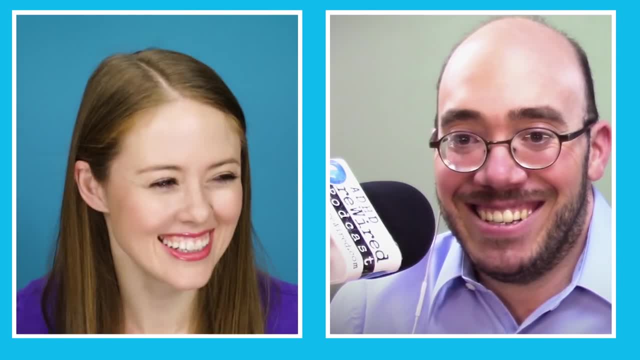 A prison. So there are two things that I just saw and heard. One was next question: please, I don't even know how to answer that. And the other thing: there's always some kind of-. I don't even know how to answer that And the other thing is okay, but in the end, if I don't 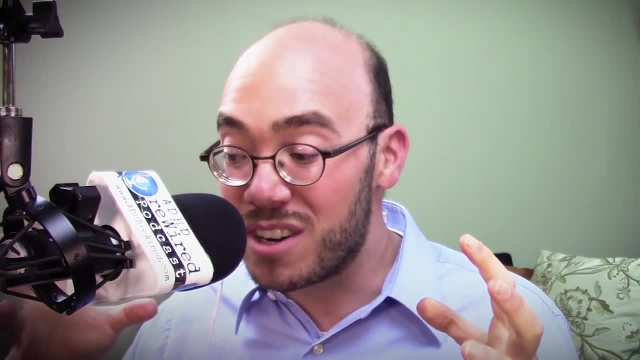 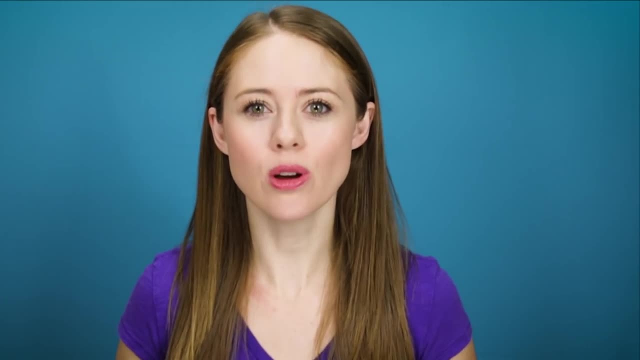 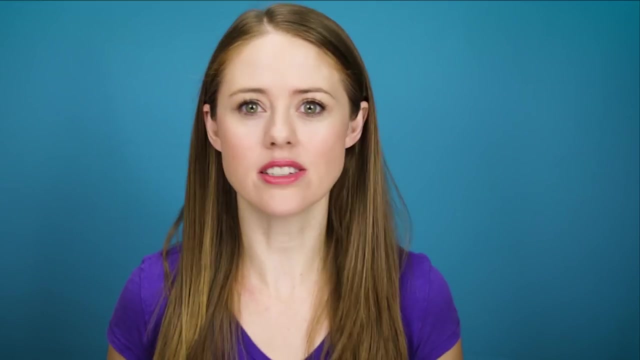 that and the the other is like: this is so, you know, constraining, I don't want to schedule. then I have no ability to have spontaneity. that's what I'm afraid of. I am so afraid of not having any spontaneity in my life and that's gonna make me less fun or less interesting. I have such a hard. 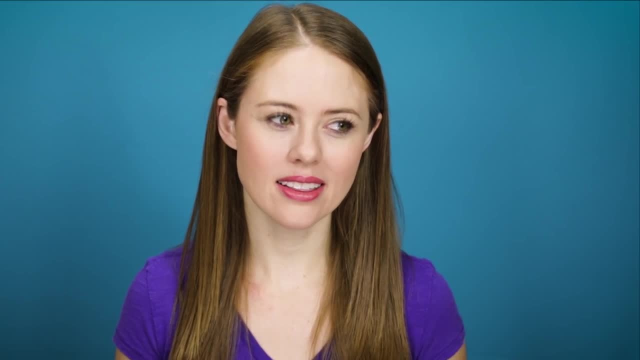 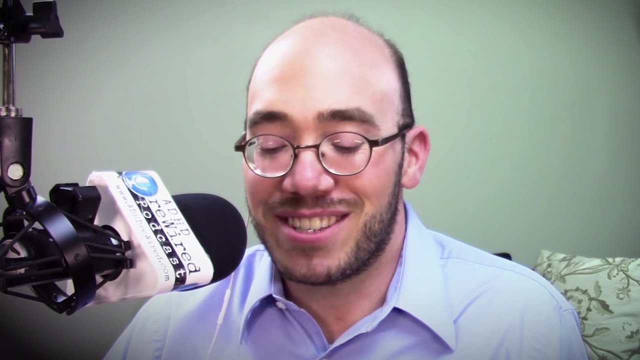 time sticking to a schedule that I end up being like the schedule police for the other people in my life. anything that feels like it might throw me off schedule stresses me out. do you think that there's? there's also an element of you're overwhelmed and sort of getting laser focus. 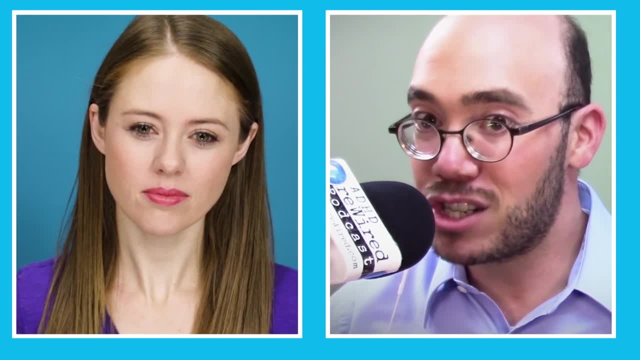 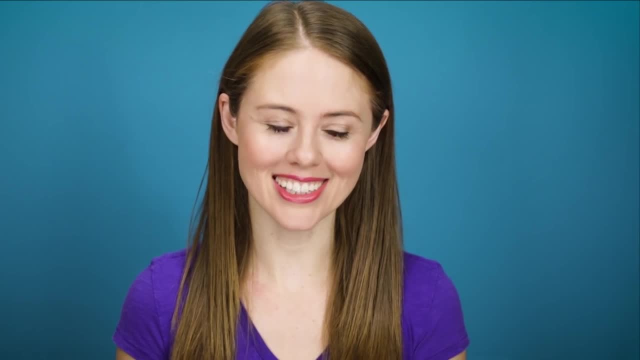 where you're kind of like you know, but anyone's interrupting with your schedule, partially because you haven't had a schedule to now. you're at this point. I mean that's part of it for sure. right is, by the time that I sit down and make a schedule, it's because I need one when you make a schedule. 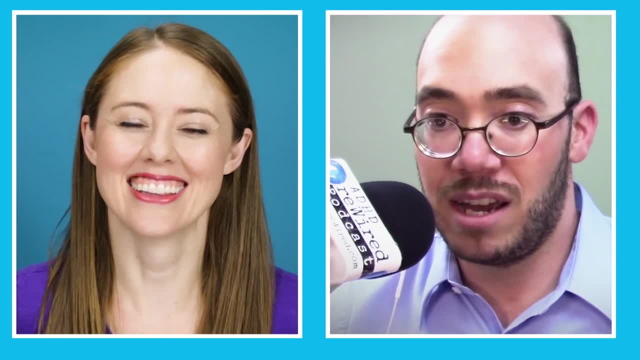 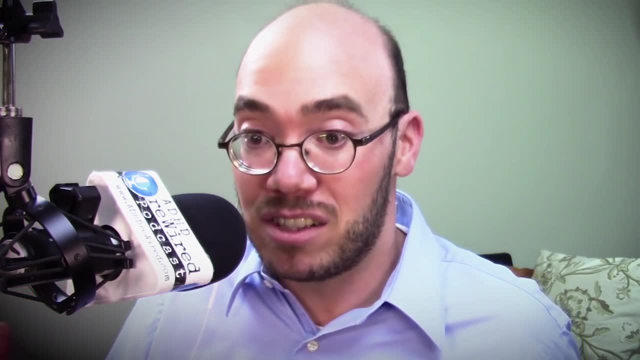 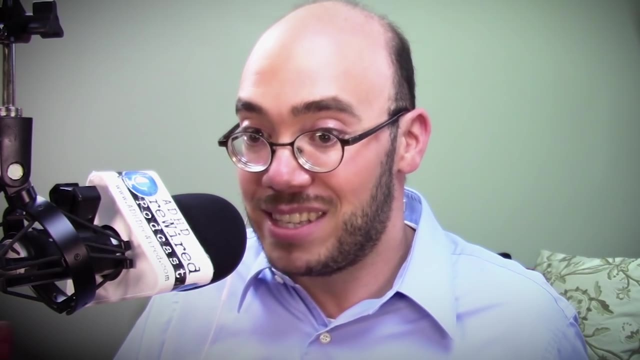 for yourself. do you get like a big slab of stone and a chisel? I mean not generally speaking. okay, I mean that's, that's good. I'm glad to hear that, because schedule or calendar is a tool that allows you to have flexibility, to create flexibility, let's say something else comes up. you can take that thing that comes up and say, hmm, this is what. 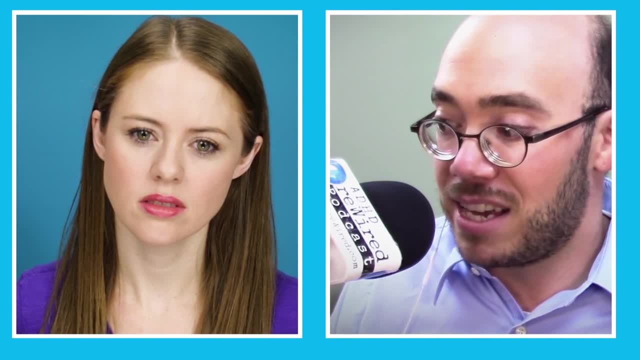 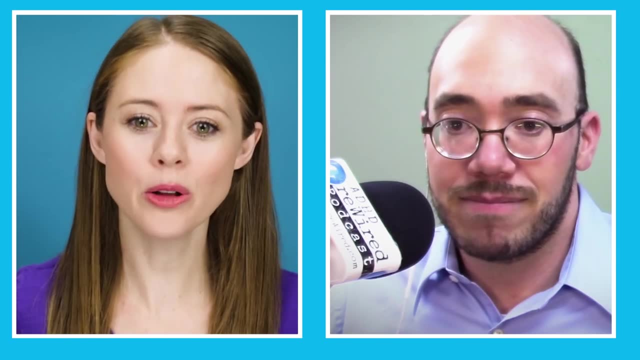 I was planning on doing, but I'm looking ahead for the next two days. I could actually do it this time, and if, for some reason, that doesn't work, I also have this time that I can do that. then here's my question: how do you even begin to create a schedule? I don't understand how long my creative 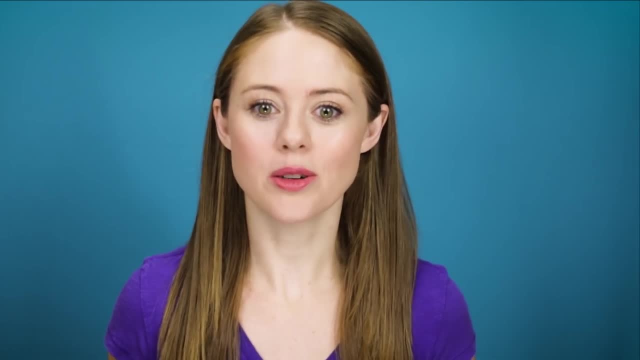 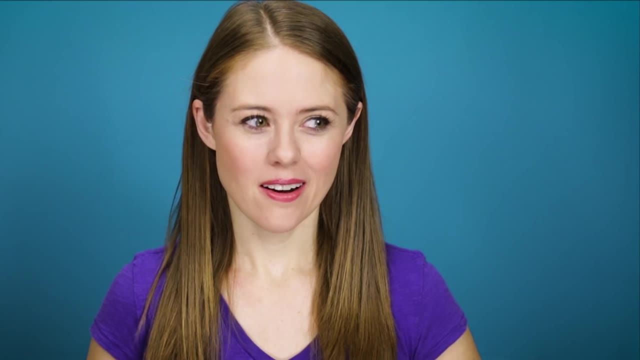 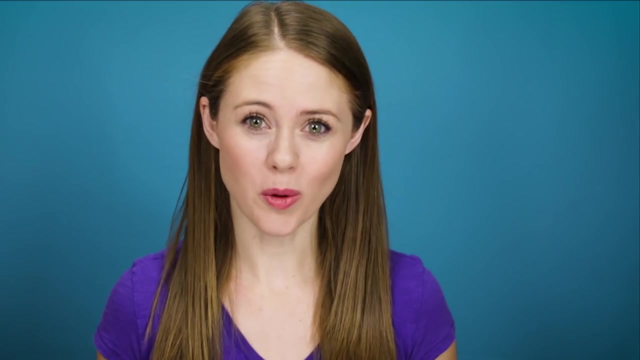 tasks will take. they could take a day, they could take five days, and I just don't know- and I'm gonna realize this is my aversion to schedules- is it's so many opportunities to fail if I don't set myself up for these are the things that I'm going to accomplish, and this is when 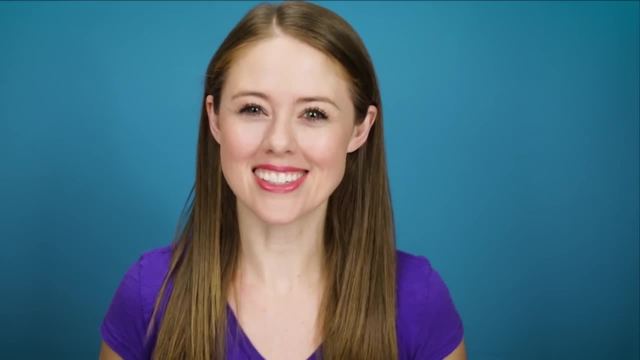 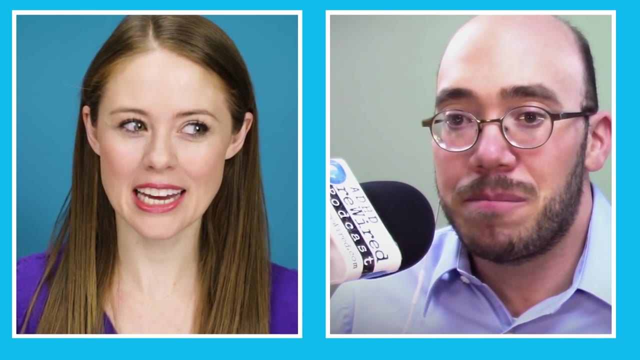 then I can't fail. anything that I do that day is a success. as soon as I have a schedule, I can fail like. not only can I, but I do constantly throughout the day, and it's it just makes me aware of of my deficits. I like to think that there's no such thing as failure. there's no such thing as failure, there's a. 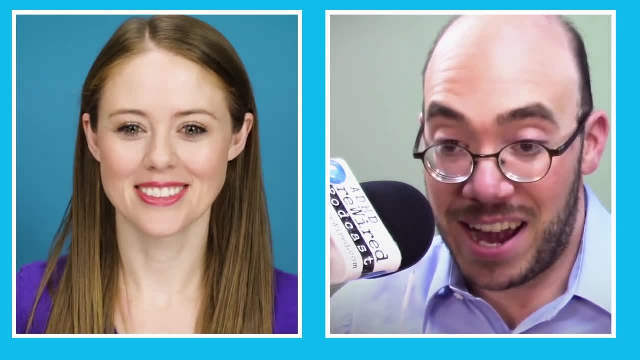 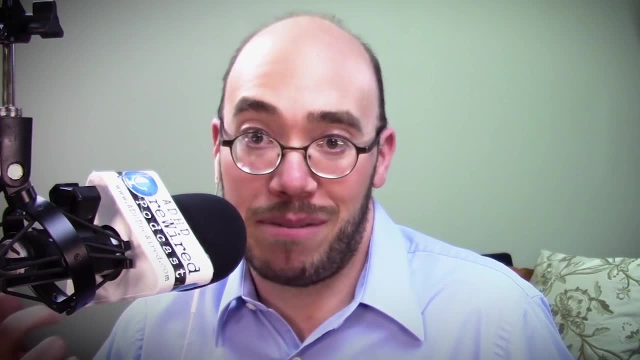 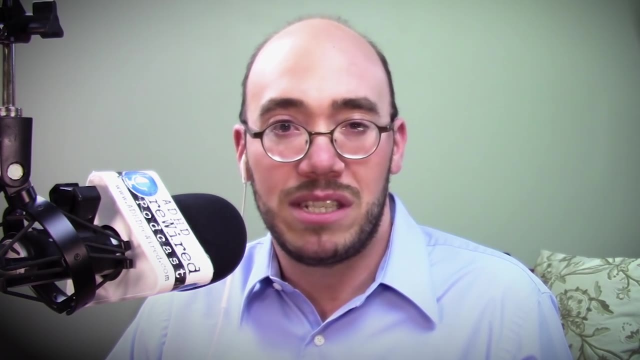 there's success and there's learning right. easier said than done, though. right as people with ADHD, we have, unfortunately, a very our. our sort of resume of failures is as bigger than we want. so there's a lot of shame. yeah, that's involved in that. it's understandable where there's a sort of resistance. 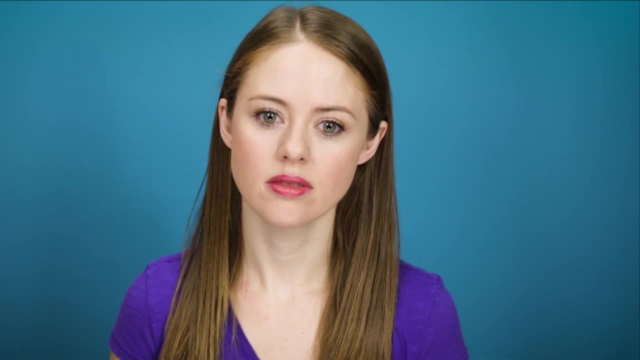 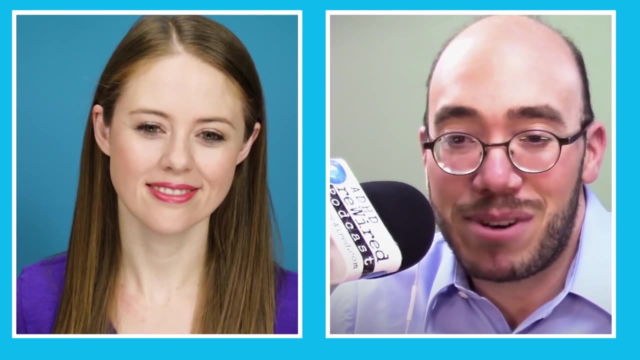 to it, because why would you want to continue to set yourself up to fail itself? one of the the things that I think is true for a lot of us with ADHD is our sense of time is pretty lousy. right, you're like, oh yeah, that'll, that'll take me 10 minutes, and that task is never taking me 10 minutes. 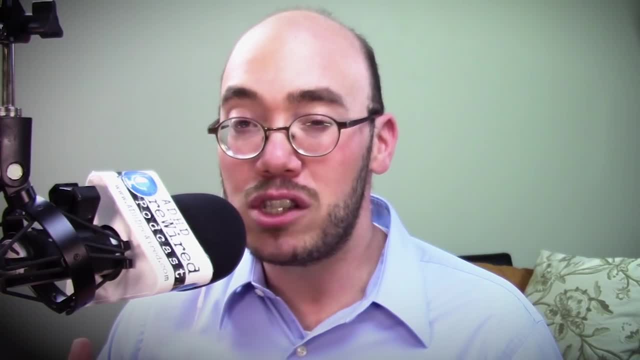 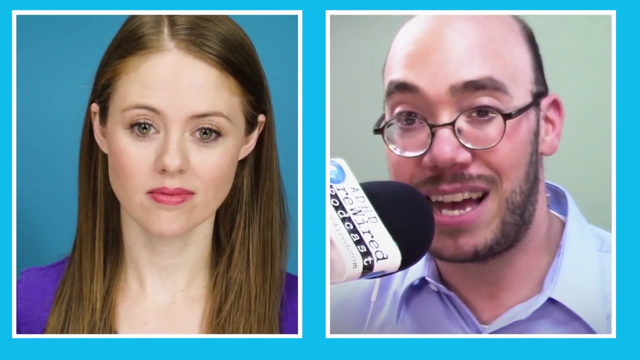 ever right, ever, ever, ever, ever. and so if you start just jumping into doing weekly planning but you're using your old sense of time, you know the part that tells you those 15 minute tasks will only take you five minutes and the thing that you think will take you half an hour actually takes a good 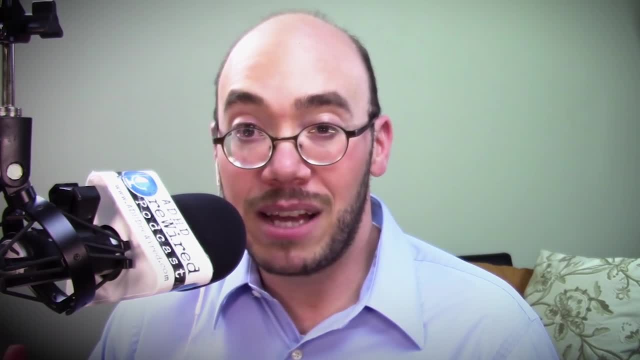 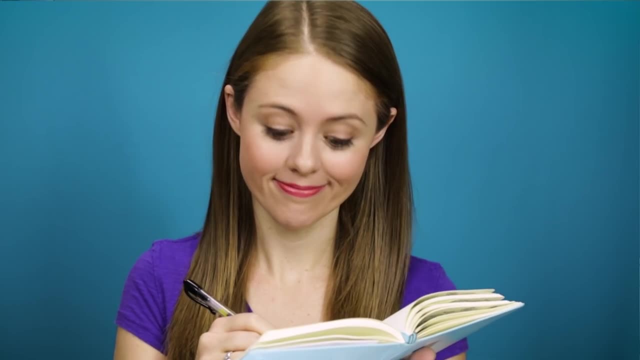 part of a day, you're gonna always feel overwhelmed because you're gonna always have too much on your plate. so the first step: if you're trying to build something big- so whether it's a youtube channel or trying to structure your home- you're trying to build something big. you're trying to build something. 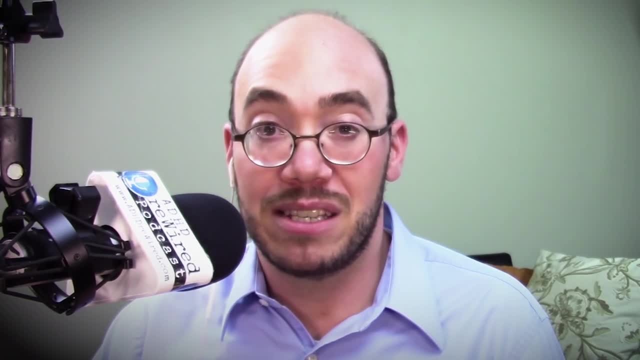 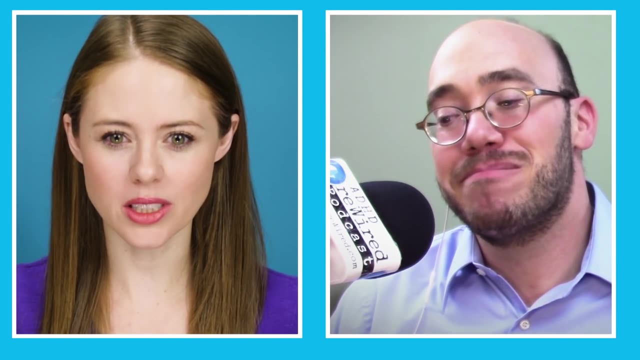 big. you're trying to get through college, like whatever it is, the first thing you have to know is: how long do things actually take you? so is that what you would recommend? like, before I try to make another schedule, would you suggest that I go for a couple weeks, timing my activities first? yes, so. 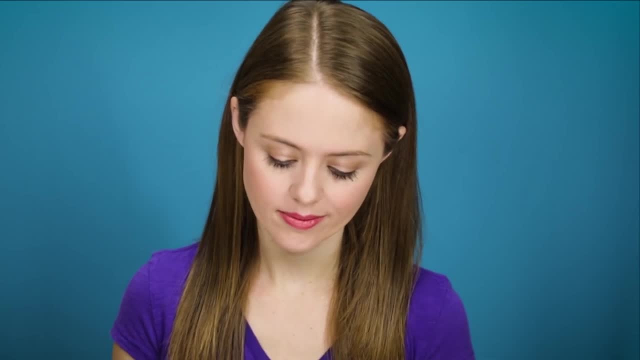 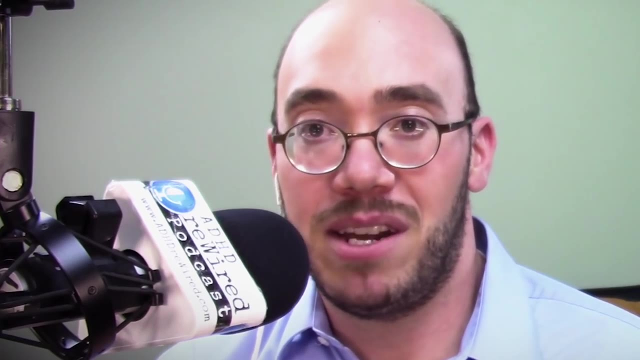 what you want to do is to take out your standard to-do list, have your task written down, and then look at the task and say: how long do I think this task is going to take me? say it's writing an email. it's going to take you five minutes. so what you do then is set a timer that actually goes up. so 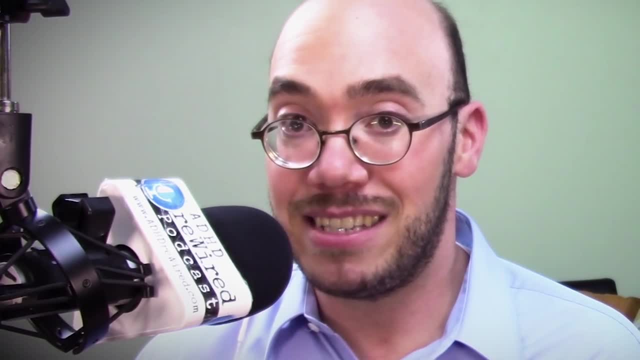 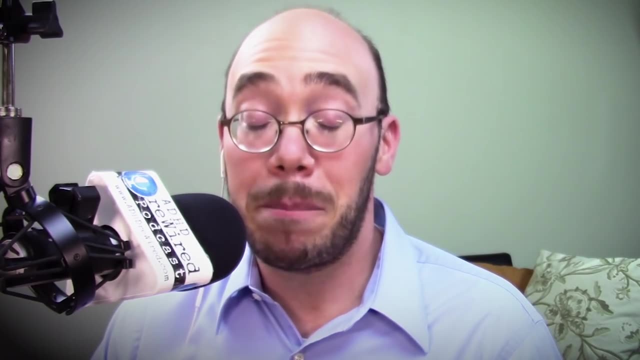 if you set a countdown timer, because if you set a countdown timer and it gets to zero and you're still working on that email, how are you going to know how long it actually took you? so you say a count up timer, stop the timer when you're done with the task and then write down how long it. 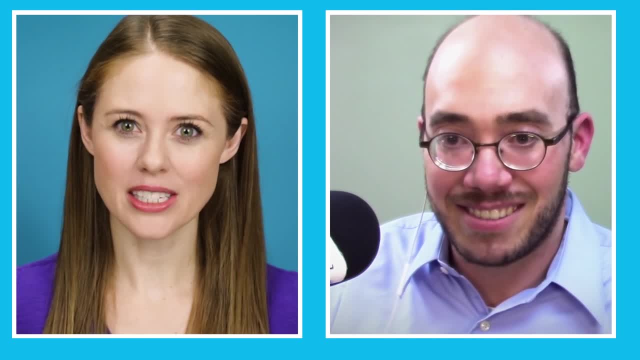 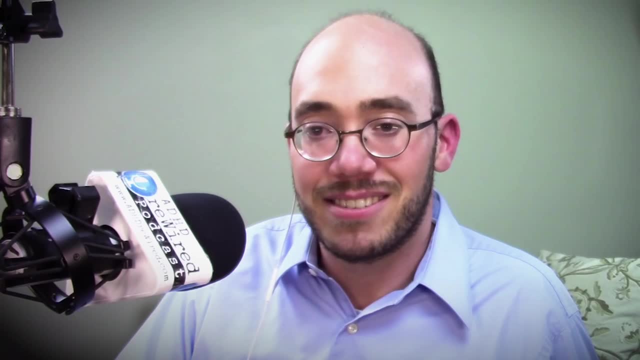 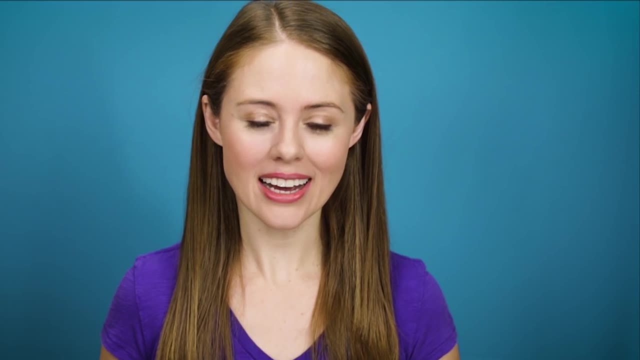 actually took you. so one of the things that I learned at the chad conference, where Eric was speaking, he said something really, really profound that I had never considered before, which is that things take the time that they take to do, but they also take prep time and cleanup time. yes, and I don't think I'd ever considered that in my entire adult life. 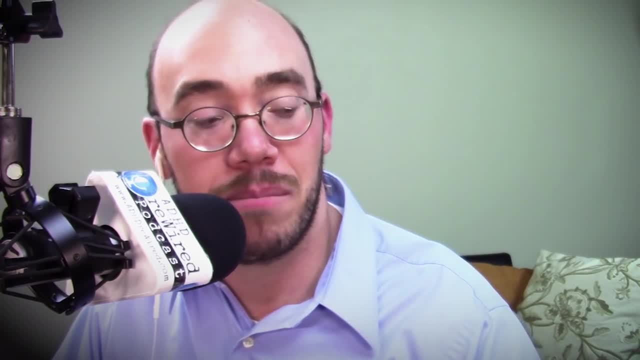 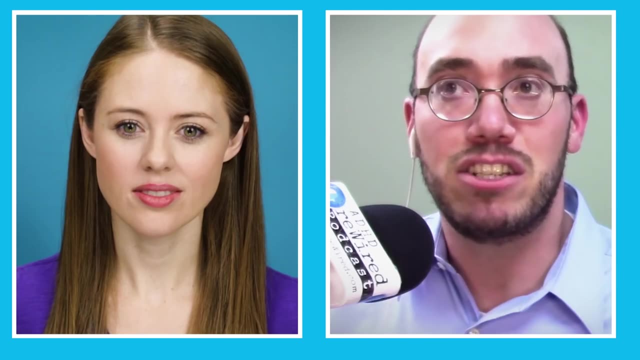 for your viewers, if you're, if you're looking around you and you're like man, these piles, they're out of control. here's the secret to this, and I learned this actually from a conference that I went to. it was talking about play. there's three parts of play: there's setting it up, playing and 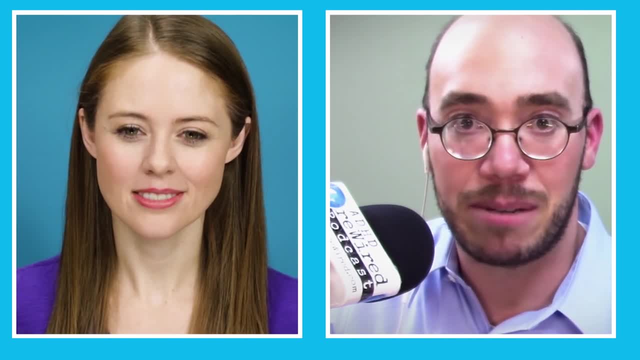 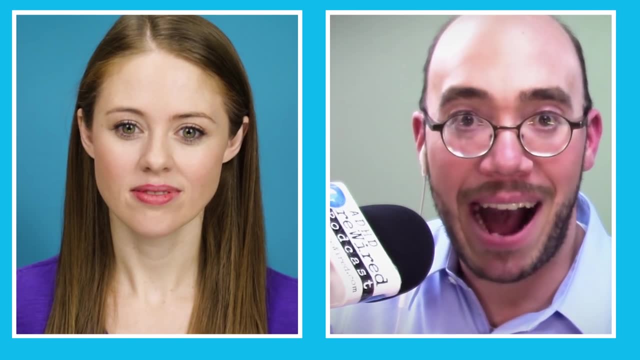 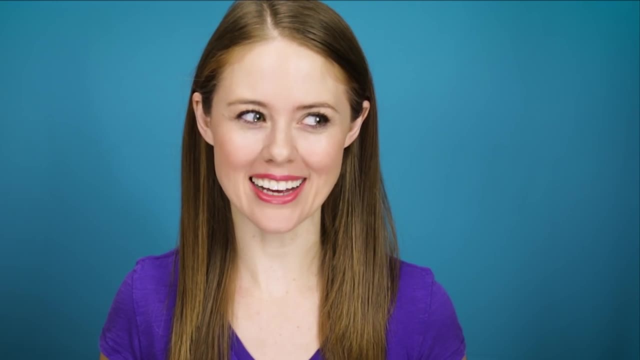 cleaning it up and I immediately made that be that connection between works the same way and I haven't been factoring in my my cleanup time and that's why I have piles everywhere. so apparently I've been doing my scheduling backwards. apparently, before you try to create a schedule and stick to it, you should figure out how long the things you're.